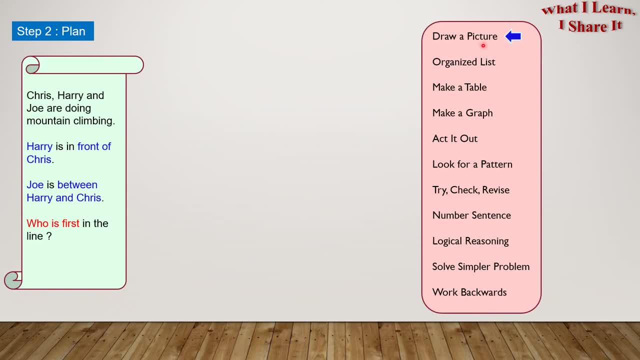 So I have chosen: draw a picture and logical reasoning. Step 3. Solve. So let's take this problem step-by-step to solve it. Chris, Harry and Joe are doing mountain climbing, So here's Chris Harry and Joe. 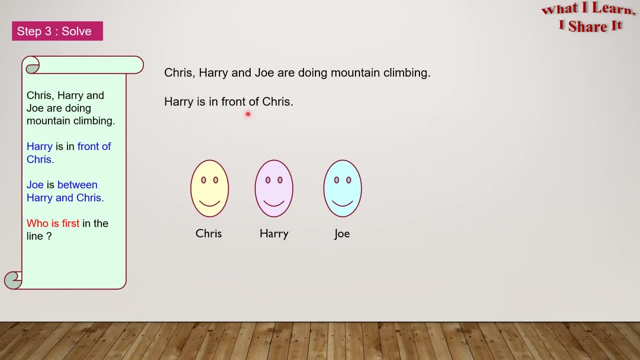 Harry is in front of Chris, So let's make Harry in front of Chris. Joe is between Harry and Chris, So let's make Joe between Harry and Chris. Who is first in line? Of course, we can see that Harry is first in line. 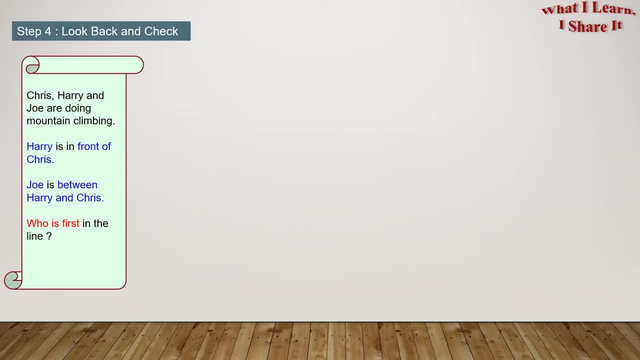 Step 4. Look back and check. In this step we check if the solution we provided in the previous step was correct or not. For this let's check if the order of the boys satisfies all conditions of the word problem. The order we found was Harry and then Joe and then Chris. 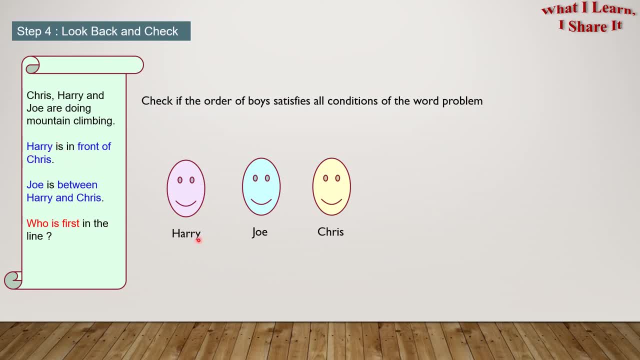 So Harry is in front of Chris. Yes, Harry is in front of Chris. Joe is in between Harry and Chris. So Joe is between Harry and Chris. So that means Harry is first in the line And that means we are correct. Do you want to try another strategy? 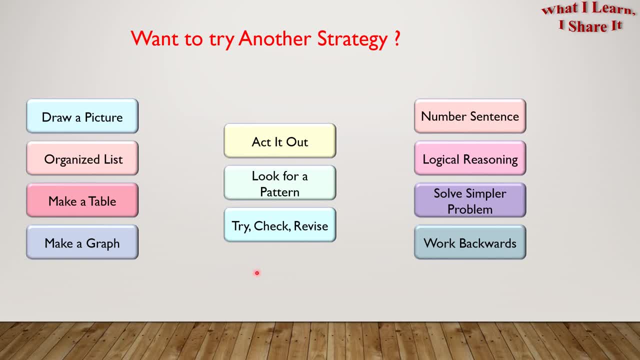 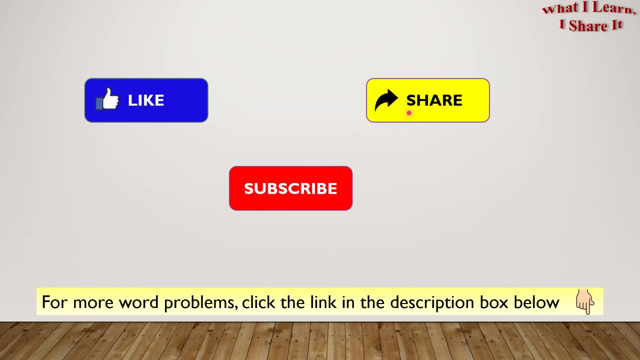 You can choose another strategy and try solving it yourself. For more word problems, click the link in the description box below. Hope you like my video. Thanks for watching. Please like, share and subscribe to my channel. See you, Bye.